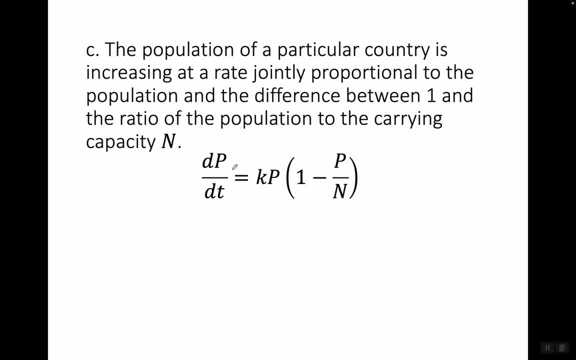 But it's cool, It does make sense and it is realistic. Okay, so this is the rate at which the population is growing: dp, dt. We're told that it's jointly proportional to the population. so jointly proportional It's going to be k times the population and the difference between 1,. 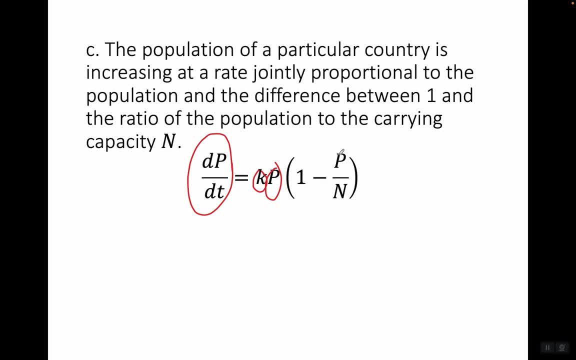 so in other words, it's going to be 1 minus something and the ratio of the population to the carrying capacity, n. So in other words, it's going to be 1 minus p over n. So p is the population, n is the carrying capacity. 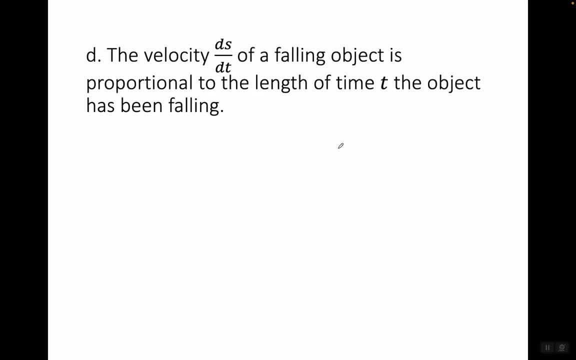 That's the maximum population possible. The velocity ds dt of a falling object is proportional to the length of the time t the object has been falling First. why use ds dt for velocity? Where does that s come from? We often use s for the position of the objects. 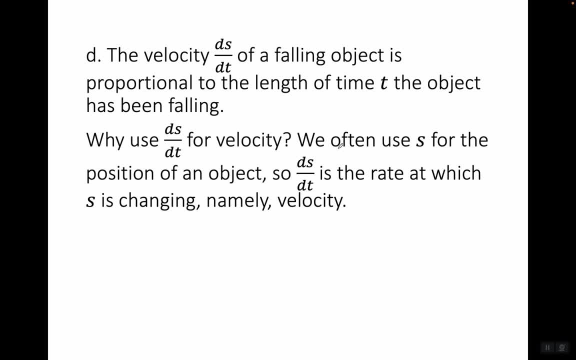 So ds dt is the rate at which s the position is changing, namely velocity. That's what velocity is the rate at which position is changing? Okay, so we end up with ds dt equals k times t, So the velocity is proportional to the length of the time the object has been falling. 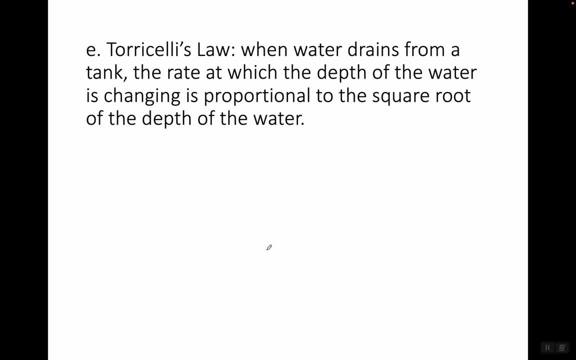 ds. dt equals k times t. Torricelli's Law: When water drains from a tank, the rate at which the depth of the water is changing is proportional to the square root of the depth of the water. And this is true. This is not just something we're making up. 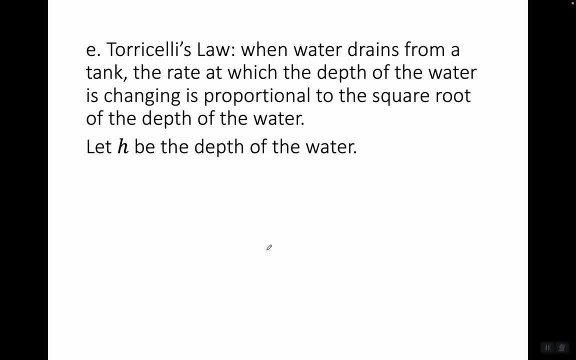 Let h be the depth of the water. I'm not going to use d for depth, because then you have dd dt and it's just kind of awkward. So h is the depth of the water. We would represent it in this way. So dh dt is the rate at which the depth of the water is changing. 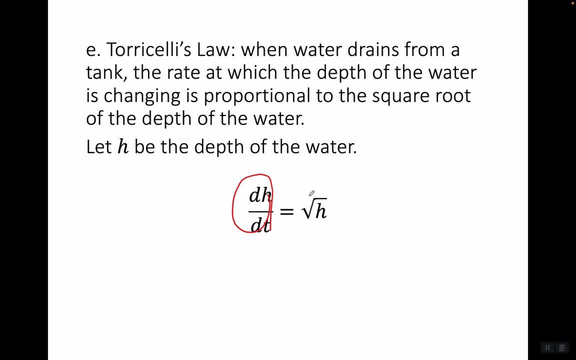 And we're told it's proportional to the square root of the depth of the water. See anything missing here? Yeah, we need to have a k here, So don't just write h or square root of h. You've got to write k times square root of h. 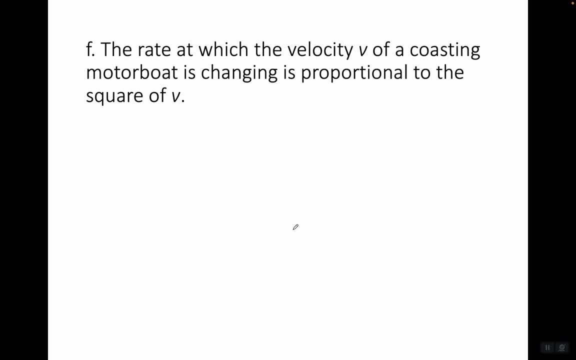 Don't forget that The rate at which the velocity is changing- The velocity v of a coasting motorboat is changing- is proportional to the square of v. This would be dv- dt. This is the rate at which the velocity is changing And we're told it's proportional to the square of v.